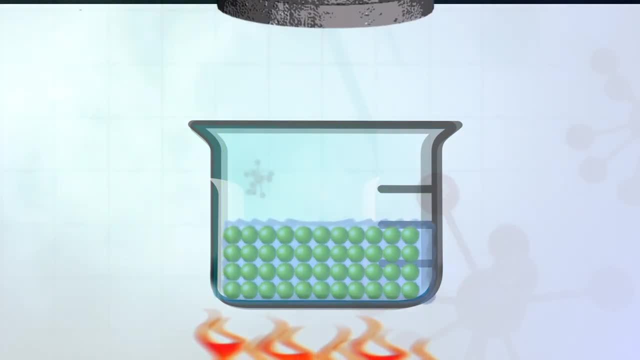 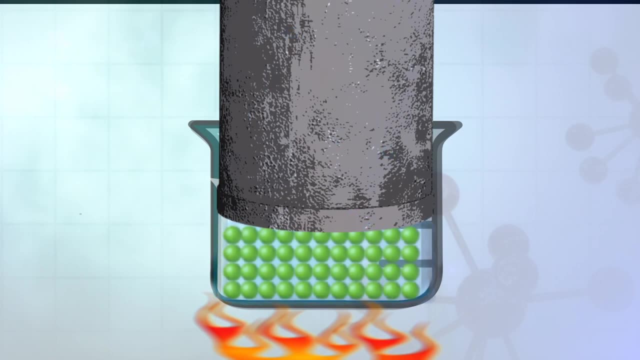 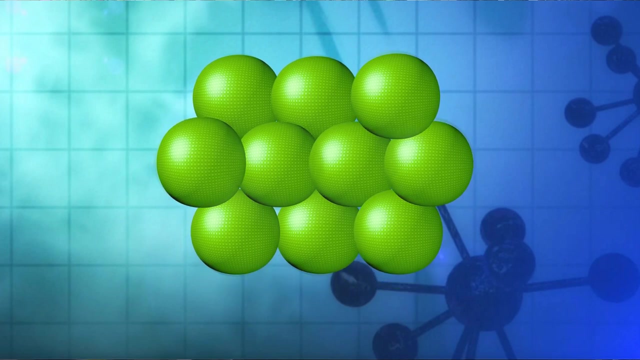 evaporation process. You're evaporating the liquid at the same time as you're dissolving it, And so you're catching this so-called dissolution and precipitation process, the crystal growth process, at the same time in and around surfaces of this powder compact, And in doing that you pick up what 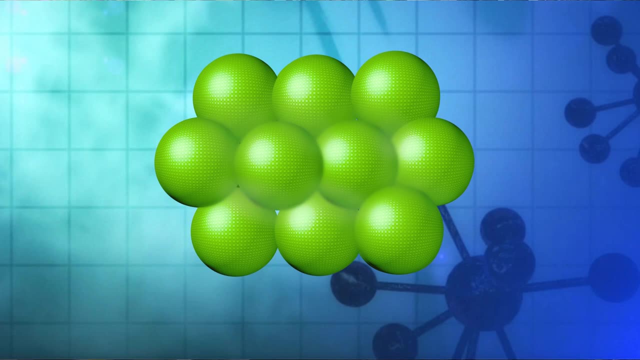 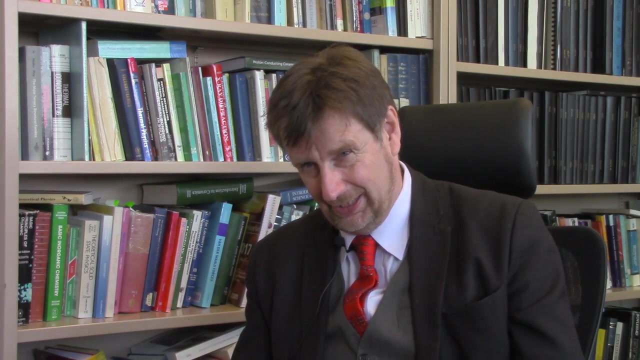 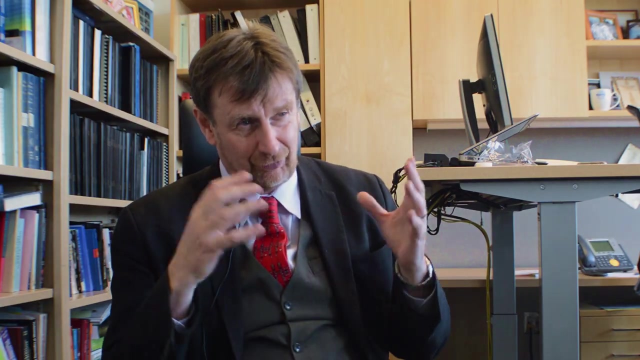 is commonly known as the liquid phase sintering process. Now, that's been done before, but usually with phases that aren't transient, And so what's really important about this process is that this is a liquid. This liquid is there and then it's gone, But in the process of it being there and gone, 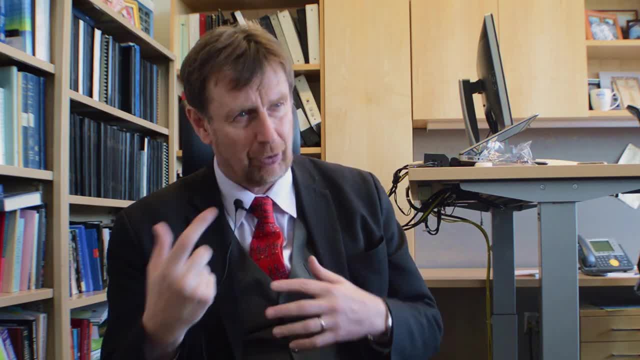 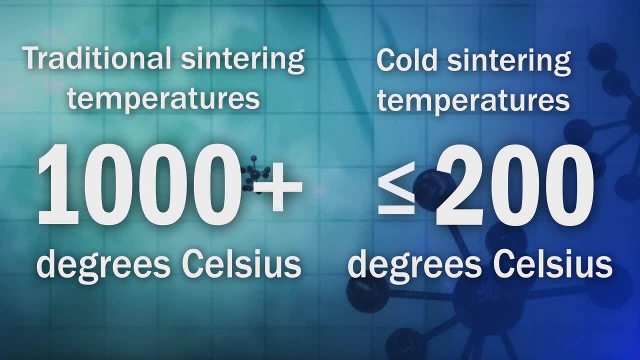 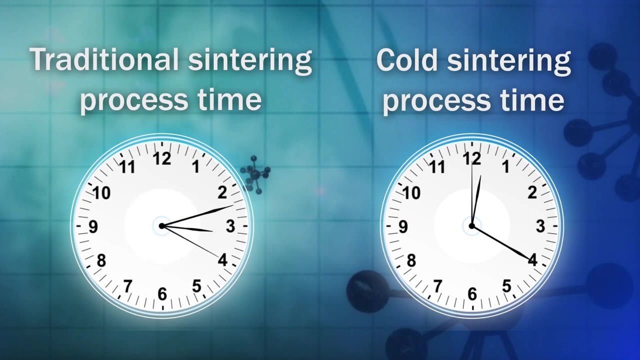 it's capturing all the exchange and diffusional and growth processes that you need to drive the sintering. This approach was named the cold sintering process because of the drastically lower temperatures needed compared to conventional high temperature sintering. This breakthrough opens up a new 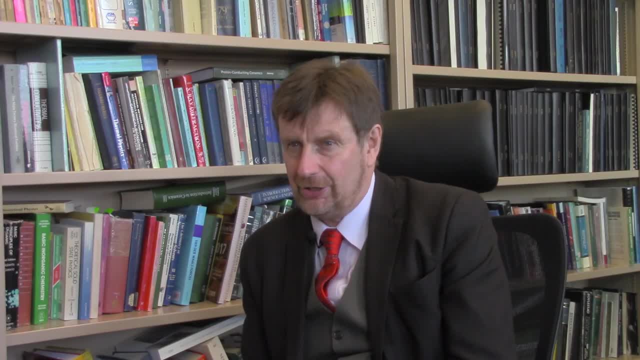 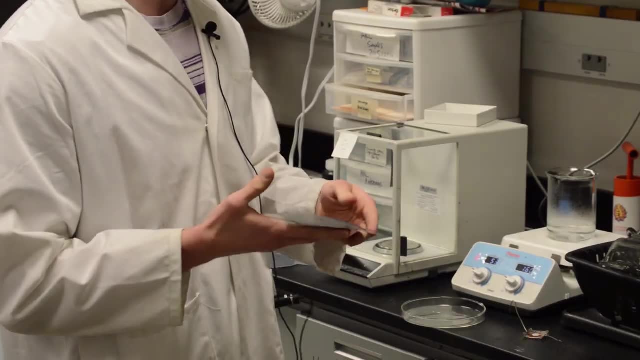 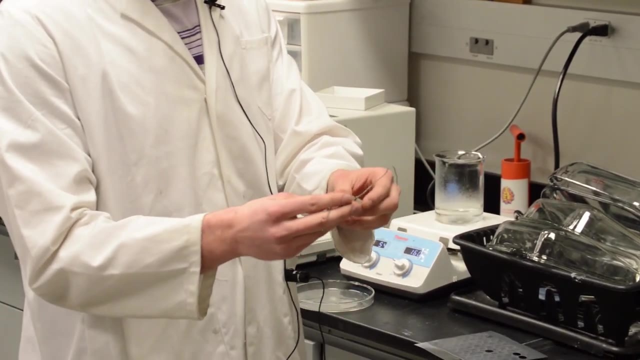 age of ceramics processing: The ability to be able to make things at the same quality that you can, that you came with a conventional process but thousands of degrees below the temperatures that you could previously do by a sintering process. the ability to incorporate new materials into that whole process and make new 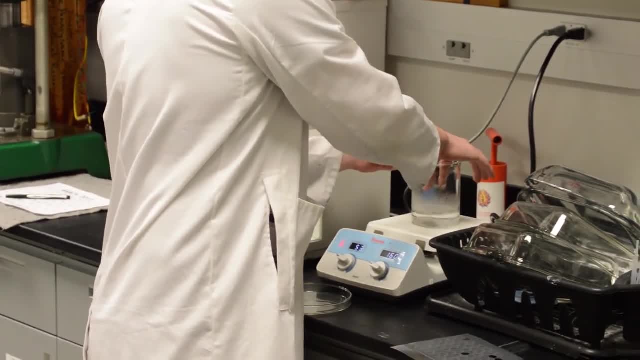 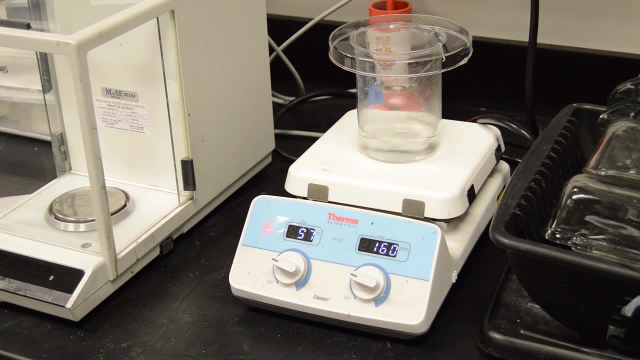 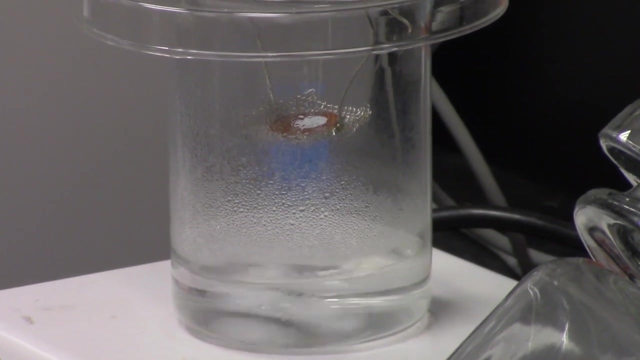 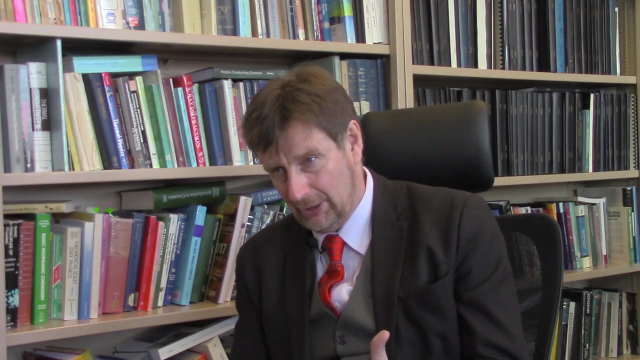 types of functionality and then finally to have a system where it's basically densified in 20 minutes means that your throughput and your manufacturing yields could go up enormously. and so this is great for manufacturing, it is great for energy savings, it is great for the environment, it is great for new 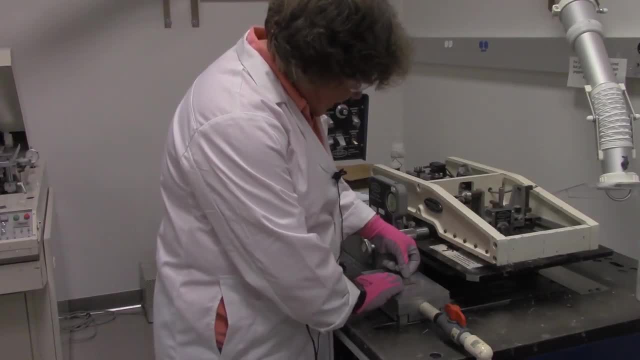 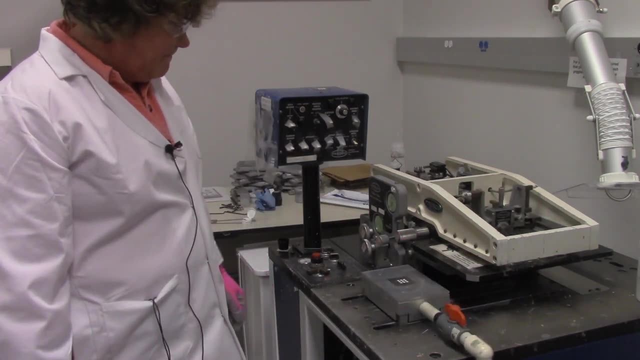 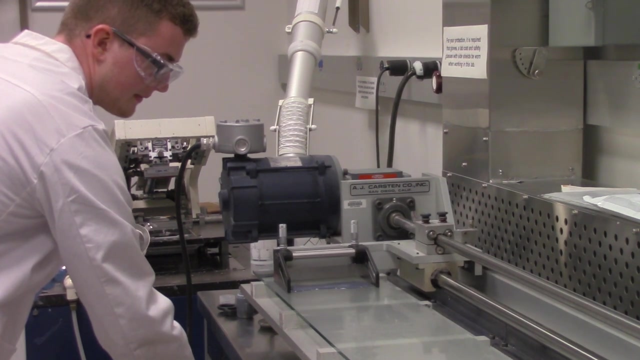 intellectual endeavors after making their initial discovery. the team has already successfully cold centered many materials. probably within three months we had worked on over 50 systems and got them all to work- dielectric materials that have very, very good properties. we're beginning to get more functional materials to work for. 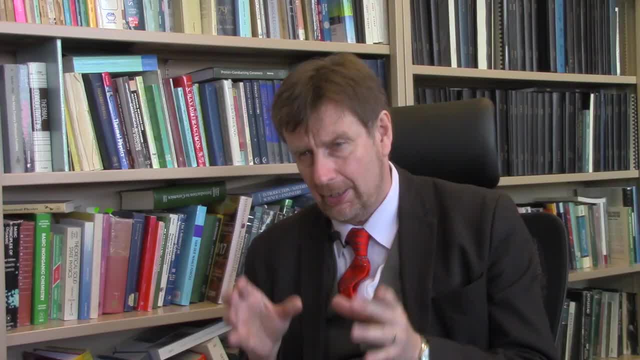 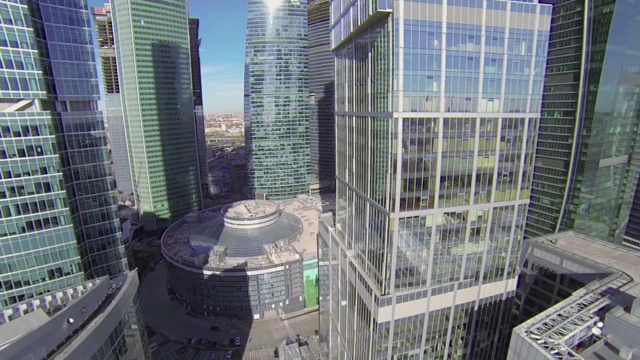 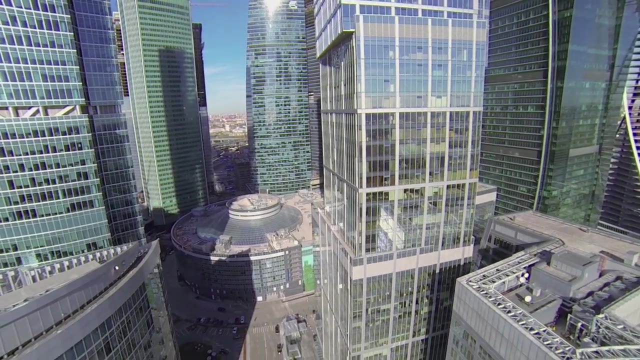 piezo, electrics and for sensors and other things like this. the real breakthrough in terms of helping the planet will be in the infrastructural use of ceramics. so this is the glass, this is bricks, this is tiles, this is this type of space through an industry, University Cooperative research.